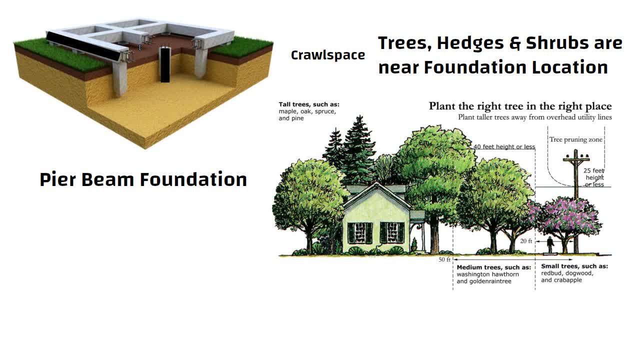 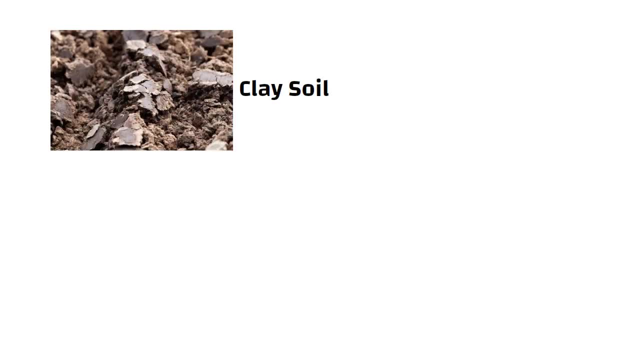 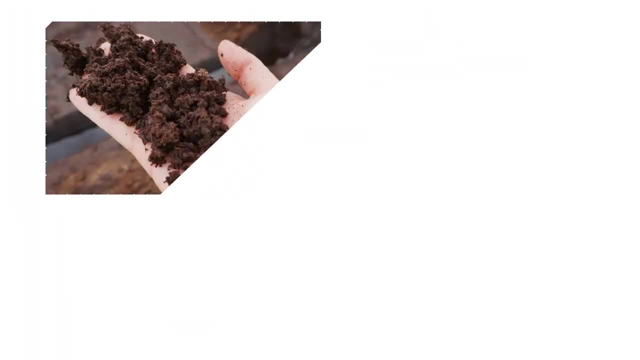 plant these trees near the structure in the future, then pile foundation carrying in situ concrete slab can be used. In short, for clay soil, wide strip foundation, raft foundation and pile foundation can be used Peat soil. Peat soil is considerably porous. 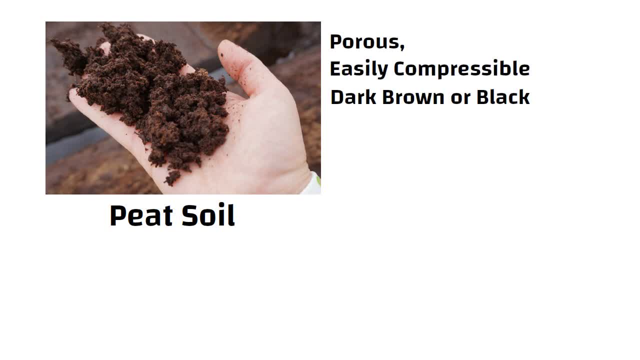 easily compressible and dark, brown or black color soil, which is commonly present near wetlands. It undergoes expansion and shrinkage due to moisture fluctuation. Extremely weak in terms of load carrying capacity, The soil can be used for a lot of different purposes. The soil can be used for: 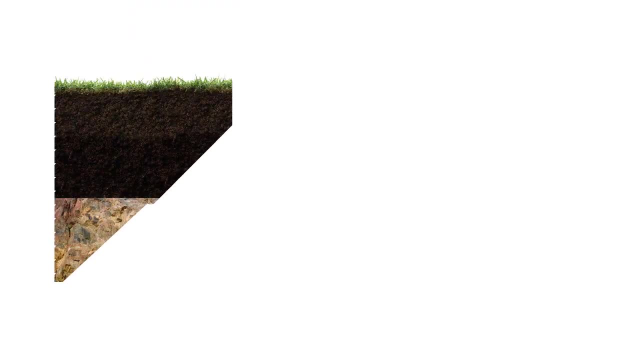 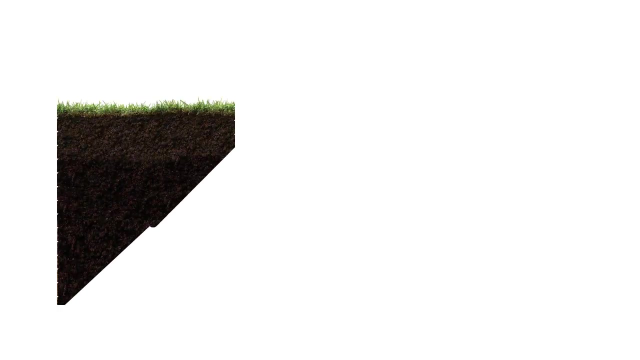 a lot of different purposes. So in some cases, when the peat layer is at shallow depth, it can be removed up to strong strata and replaced with engineered fills to build over a stronger soil, and strip foundation can be used here If the thickness of peat soil is great and its removal is not economical. 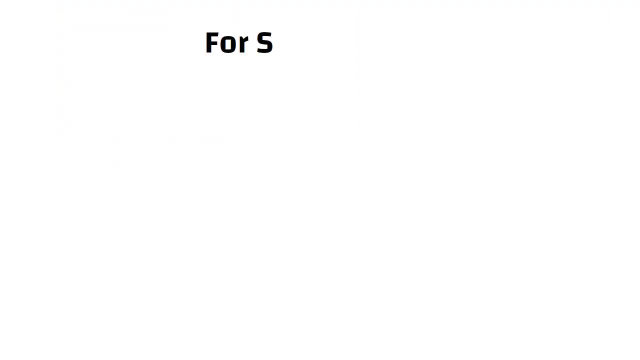 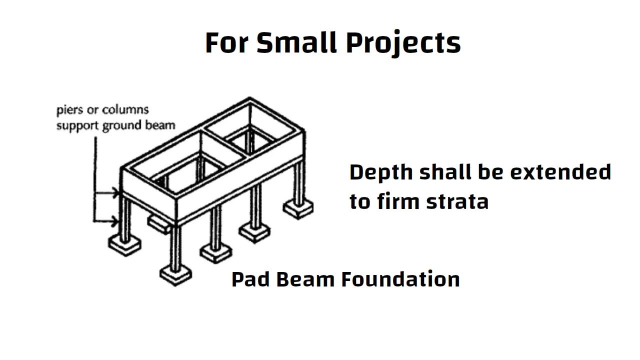 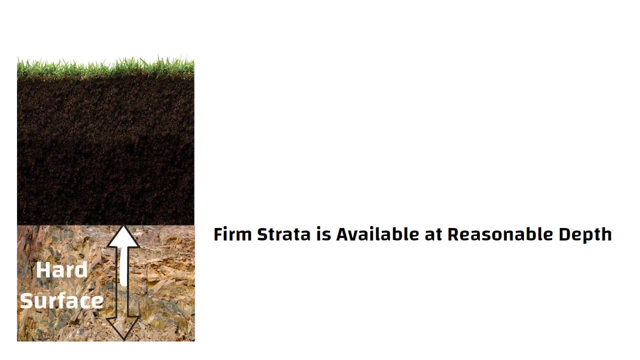 then pile foundation should be selected. For small projects, pad and beam foundation can be used and depth shall be extended to a firm strata below If firm strata is not available at reasonable depth but there is a hard surface crust with 3-4 m thickness of suitable bearing capacity. 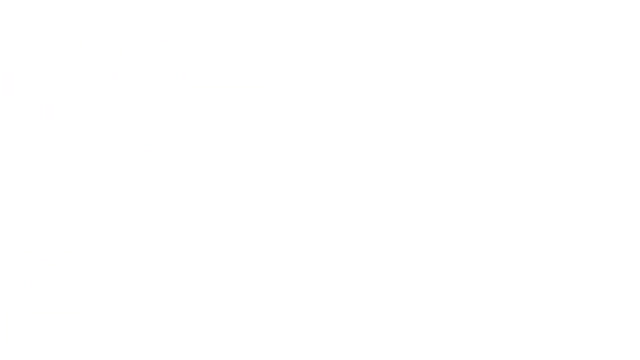 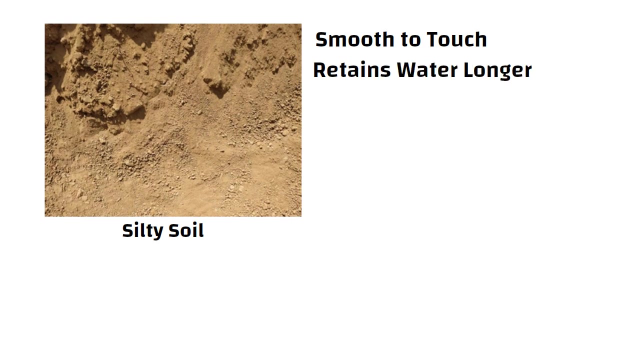 then raft foundation can be used here. Silty soil can be smooth to touch and retains water longer. because of its smaller particles, It is generally not suitable for foundation structure because of its expansion and shrinkage. It is generally not suitable for foundation structure because of its expansion and shrinkage. 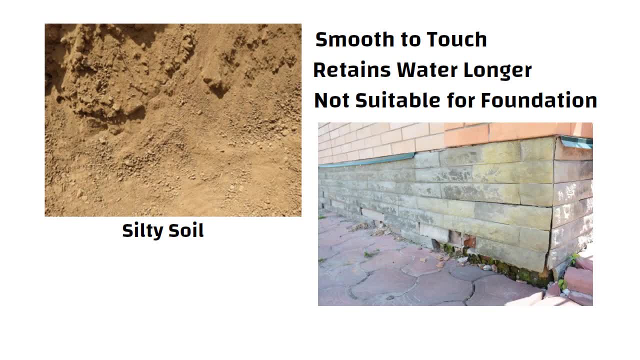 It is generally not suitable for foundation structure because of its expansion and shrinkage, which exert pressure against foundation and damage it. The silt retain moisture and does not drain water easily If firm silt or firm silty clay deposit extending to a great depth is available. 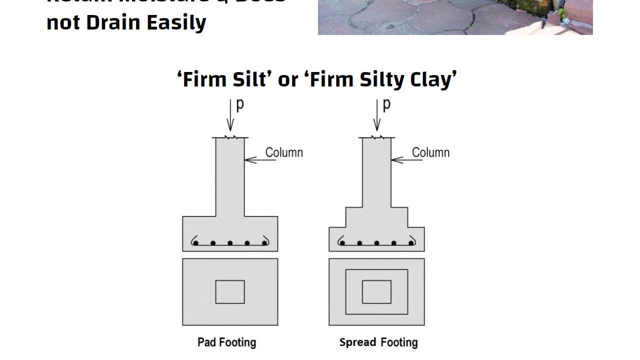 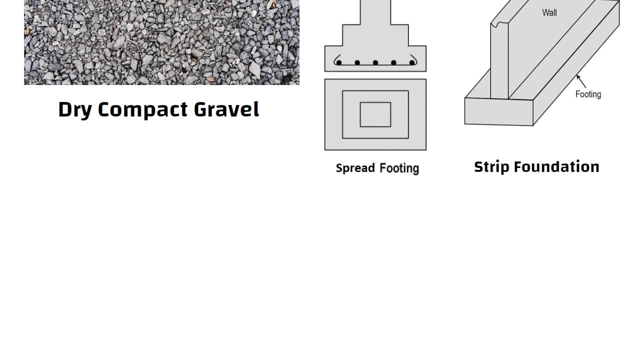 then RCC sprayed and isolated pad footings are appropriate. In case of dry compact gravel, sprayed and stripped foundations can be used. In case of dry compact gravel, sprayed and stripped foundations can be used. If gravel is submerged in water, the bearing capacity is declined by half. 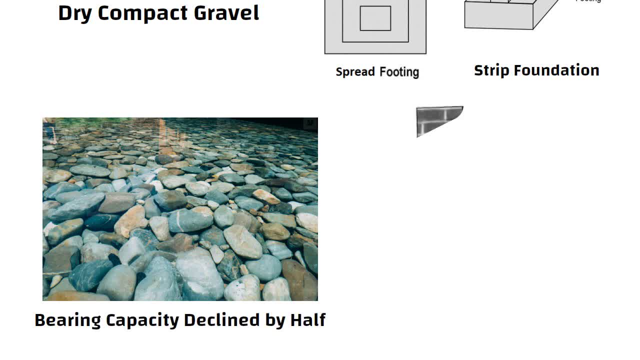 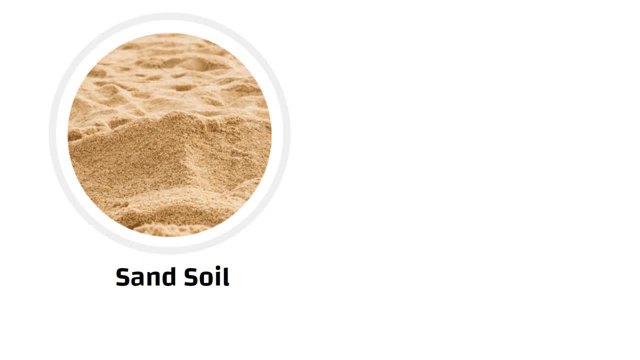 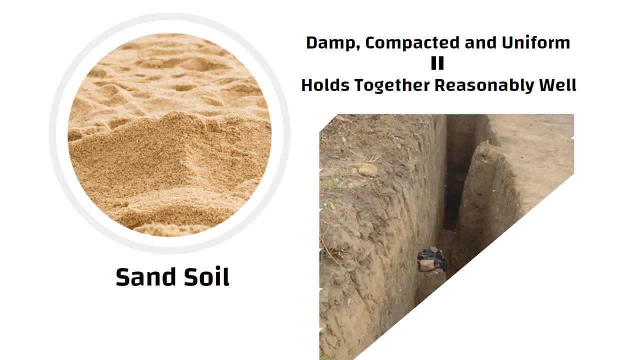 If gravel is submerged in water, the bearing capacity is declined by half. A shallow RCC white strip foundation can be used here. When sand is damp, compacted and uniform, it holds together reasonably well, But trenches may collapse. but trenches may collapse. 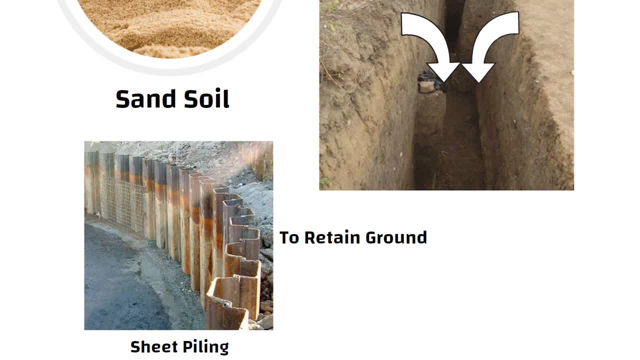 and so sheetpiling is often used to retain the ground in trenches until the concrete is poured. and so sheetpiling is often used to retain the ground in trenches until the concrete is poured. If nude sand is emitted cleanly under the sand and when it isاخ ed with foreign перед sand or added water. 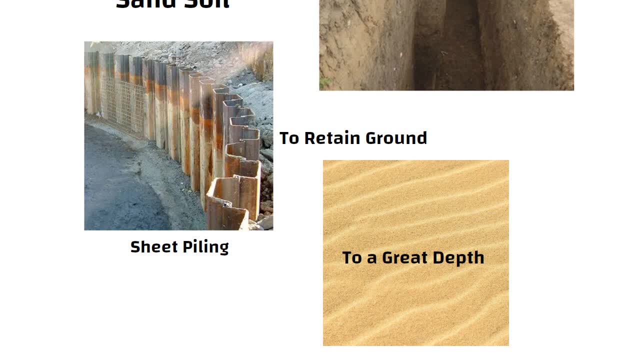 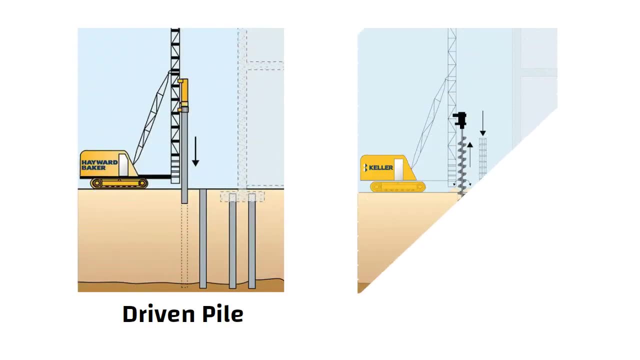 Then it old school sand, is washed away. If sand used for use it will give just – small –, solid and moisture preference extended for great depth, then it is recommended to compact it and use spread footing. Alternatively, raft driven pile or auger pile can be selected without the use of compaction energy. 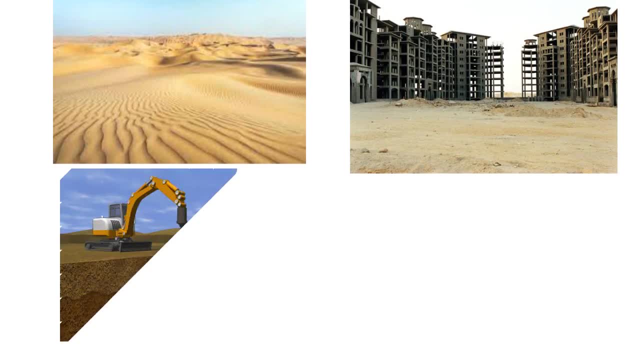 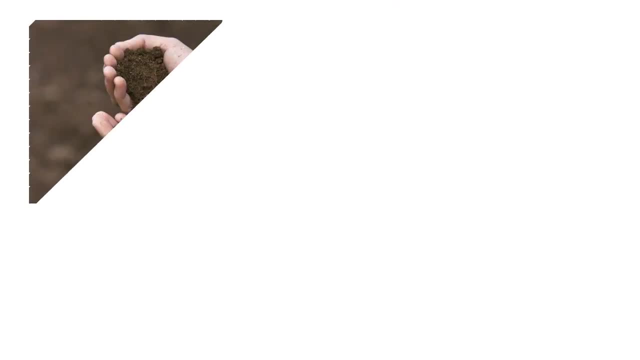 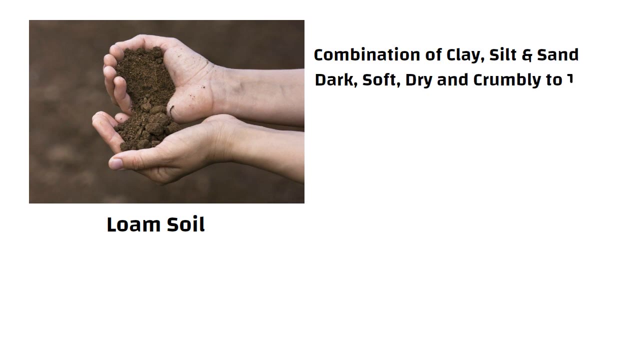 In desert soils. multi-storied buildings usually have a pile foundations, especially driven piles or auger cast-in-situ piles. Loam is a combination of clay, silt and sand. It is dark in color, soft, dry and crumbly to touch. 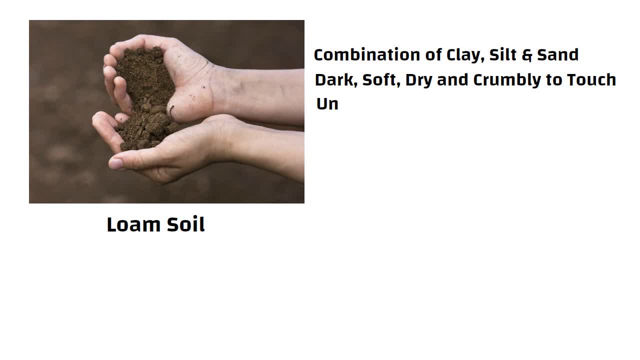 Loam is the best option to support foundation because of its uniformly balanced characteristics. It maintains water at a balanced rate and hence neither shrink nor expand to an extent that damage foundations. Isolated footing is the most desired type of foundation for loam soil. 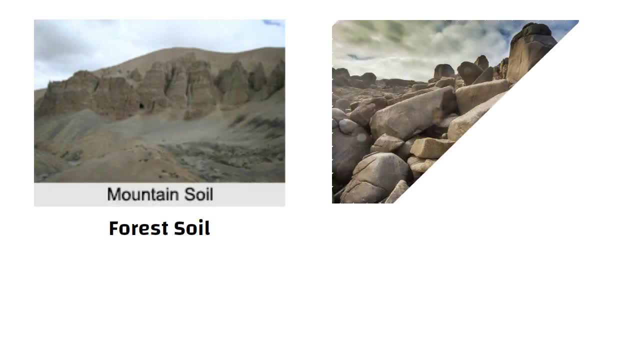 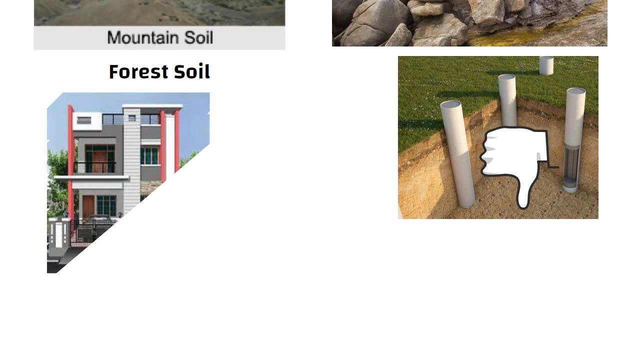 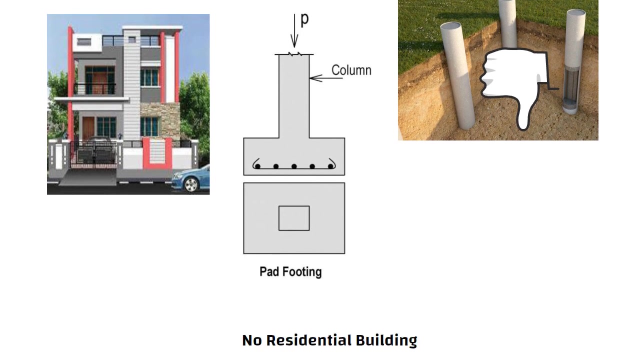 Mountain soils. Mountain soils and forest soils are most likely to have boulders at various depths, so pile foundations are not suitable here. For residential buildings with one or two floors isolated, RCC pad footings are suitable. No residential buildings should be constructed on slopes steeper than 25 degrees. 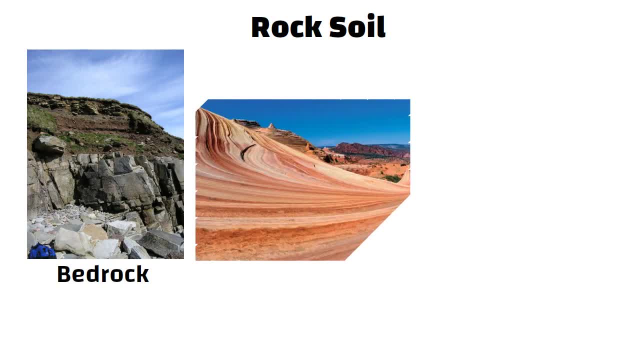 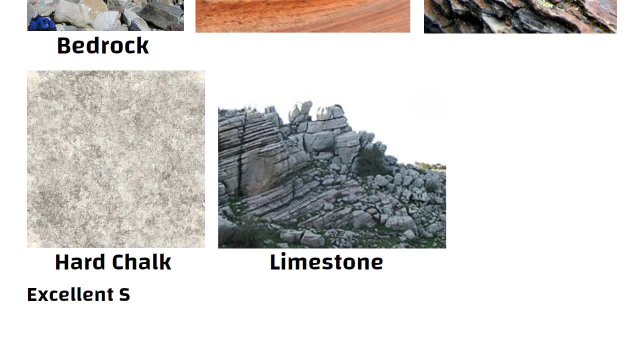 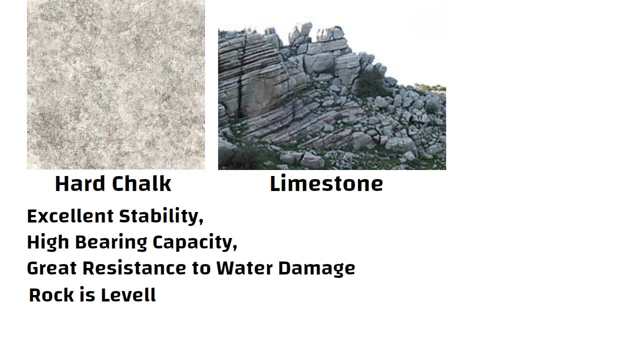 Rock soil. It involves bedrock, sandstone, shale, hard chalk and limestone. Rock soil has excellent stability, high bearing capacity and great resistance to water damage, As long as the rock is leveled and the foundation is well supported. the most suitable foundations for rock soil are strip foundation, pad foundation and raft foundation.